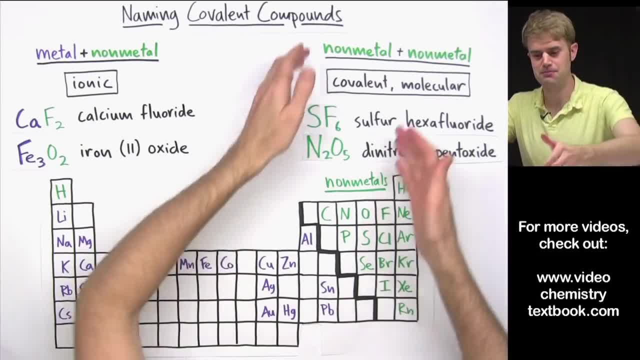 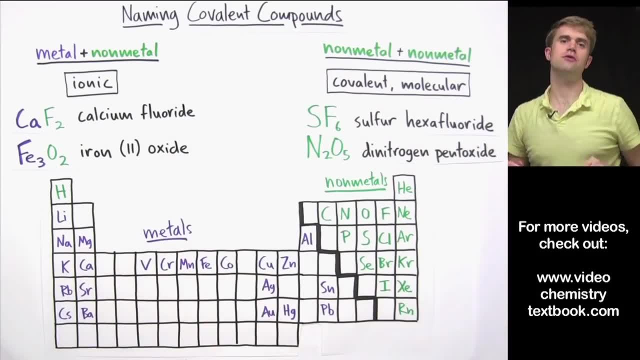 how to write formulas for them. If you need to name a compound that's made of a nonmetal and another nonmetal, well, that's a covalent or molecular compound, and naming these is what this video is going to focus on. Okay, here's our first chemical formula: N2O3.. It's made of two nonmetals We're going to 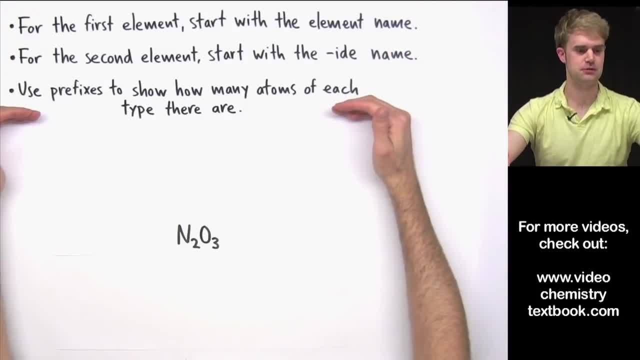 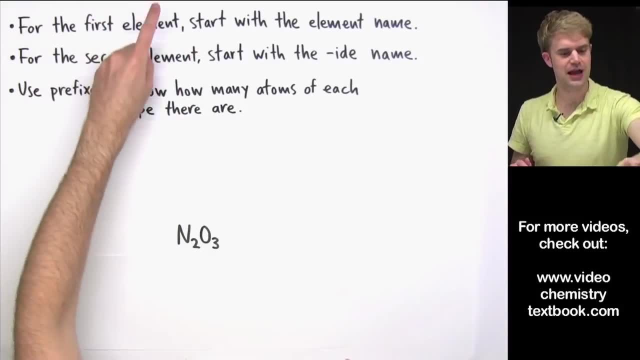 write a name for it following these steps. So here's the first one. It says for the first element: start with the element name. When I'm talking about the first element, I'm talking about the order that these elements are in in this chemical formula. So the first element. 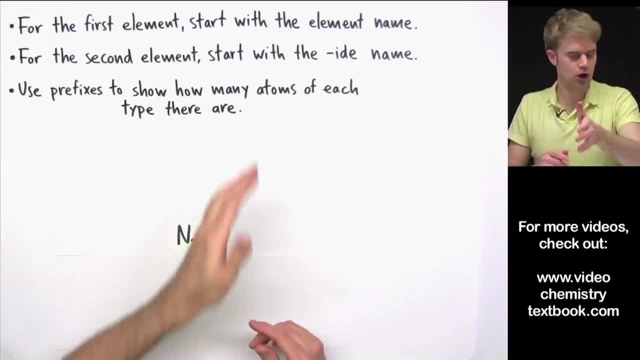 here is nitrogen N. So it says: start with the element name. Okay, so I'm going to put nitrogen down. That's the element name here. Okay, so I'm going to put nitrogen down. That's the element name here. Now for the. 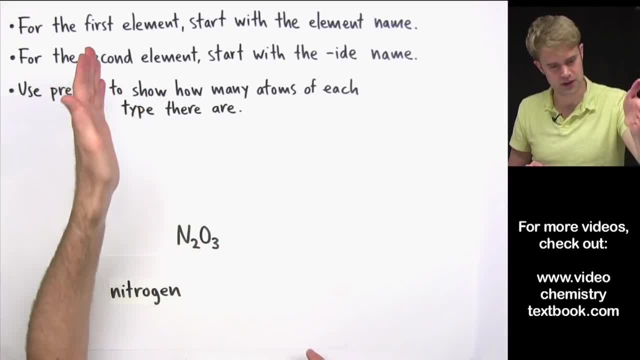 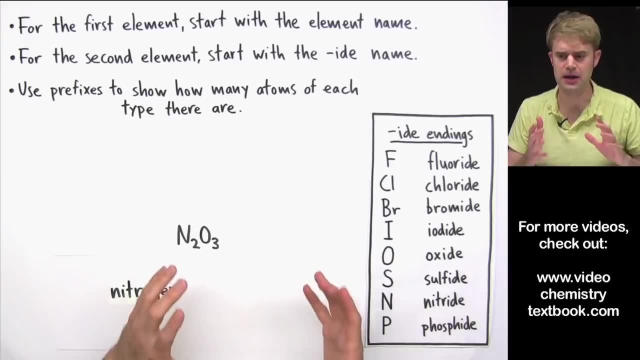 second element. so that's this here: oxygen For the second element. start with the I-D-E name. Now, the I-D-E name is the version of the element name that ends in I-D-E. These are actually the same names that we use to name negative ions. So we've got oxygen here. 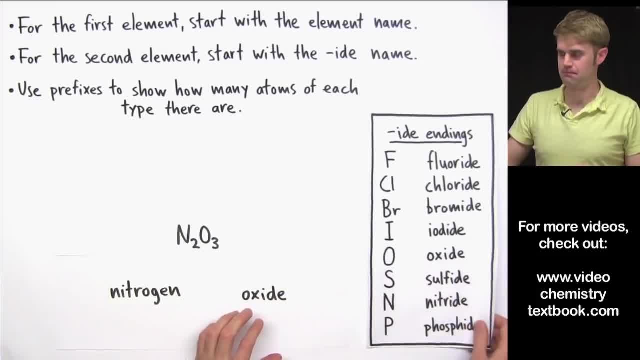 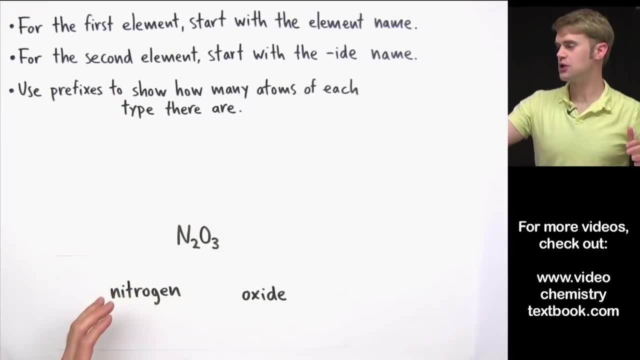 We're going to use its I-D-E name, which is oxide. Okay, so we've got nitrogen and we got oxide. Now use prefixes to show how many atoms of each type there are. The prefixes- here's a list of them- are like these little tags. 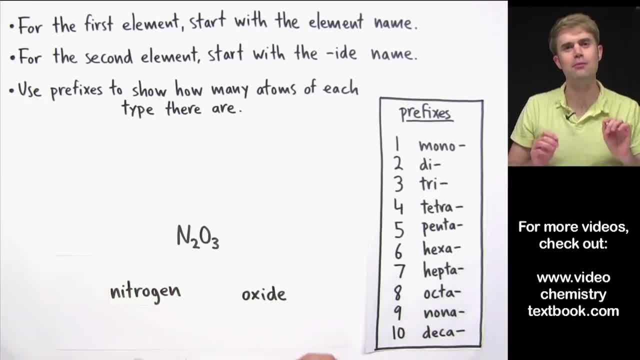 that we put on the front of each name to tell us how many atoms of each type we have. So N2, we've got two nitrogens, which means that we want to use this prefix for two di. so put that in front of the element name: dinitrogen, Now O3, which means that we have three oxygens. 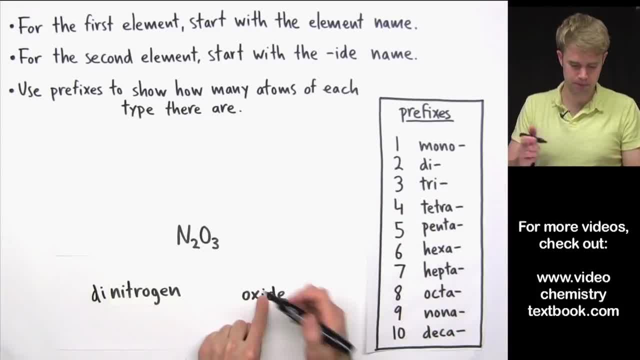 so I'm going to use the prefix tri here and write that in front of oxide, And so the name for this compound is dinitrogen trioxide. We put the element name here, we put the IDE name here and then we use the prefixes. 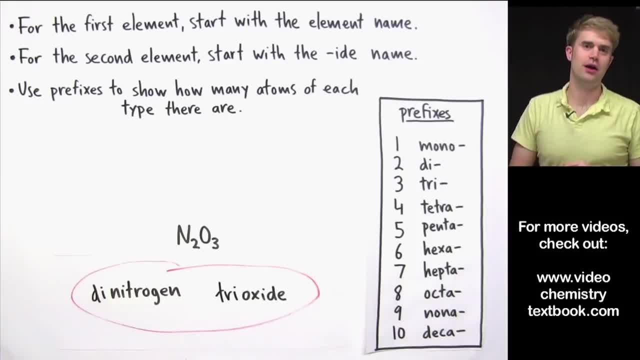 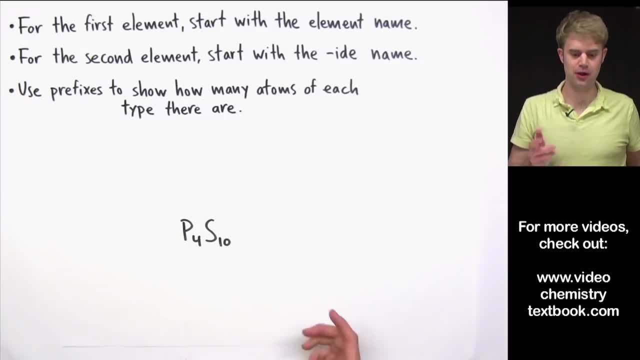 to indicate how many atoms of each type we had. Let's look at a few more examples: P4S10.. Okay, for the first element, we'll start with the element name. P is phosphorus. If you didn't know that, you could look it up on the periodic table. For the second element, that's S here. 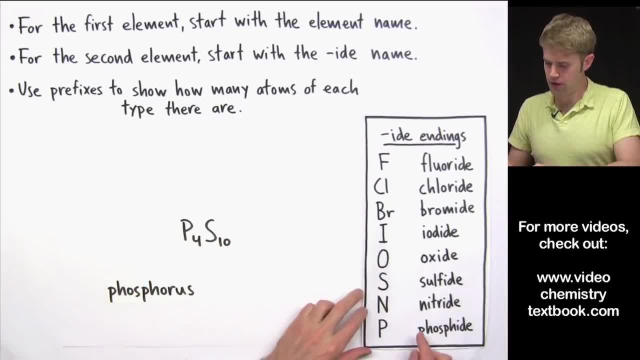 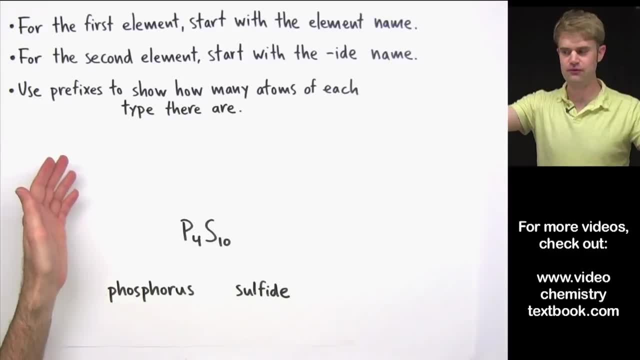 start with the IDE name. So S is sulfur and its IDE name is sulfide. Okay, so those are the two names. Now we're going to use prefixes to show how many atoms of each type we have. We got P4,. 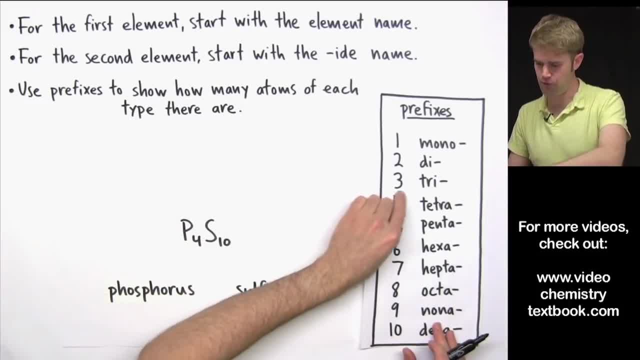 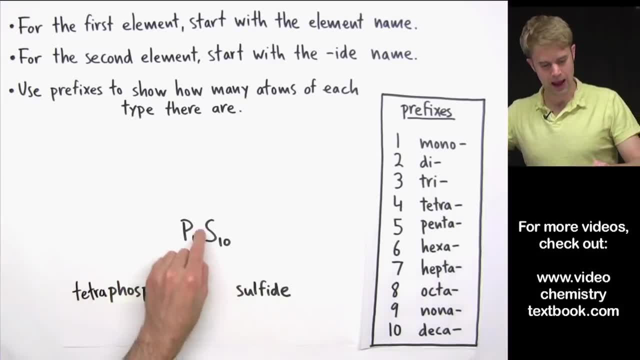 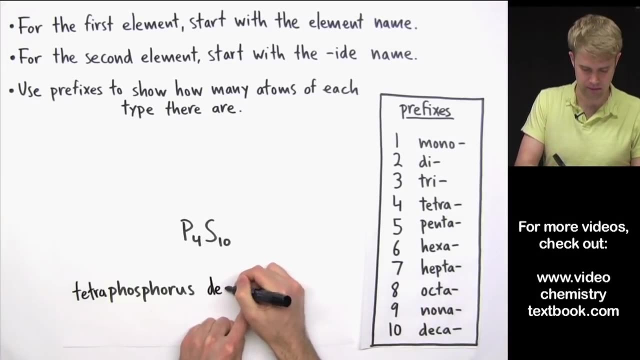 so that means we have four phosphorus atoms. So four is tetra. We use the tetra prefix, tetra, And then for sulfide we got 10.. So we'll use this prefix: deca, Deca. So the name of this compound is tetraphosphorus decasulfide. Let's move on. 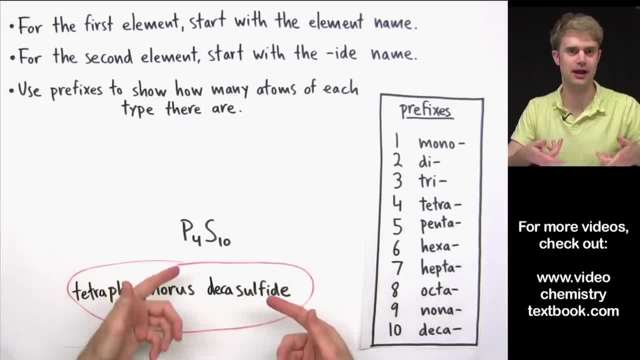 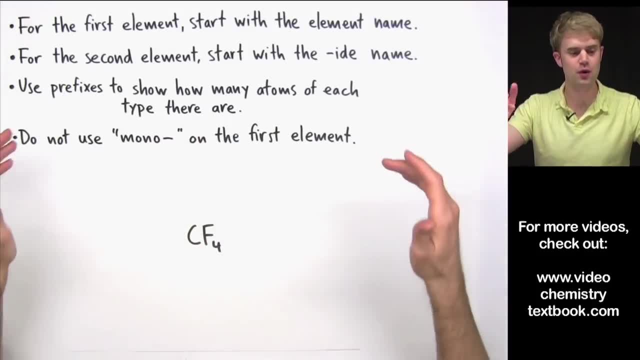 We're going to add a couple more steps to deal with more complex formulas. Here's the next step that we're going to talk about. Do not use mono On the first element. I'm going to show you what this means by working through naming this formula. 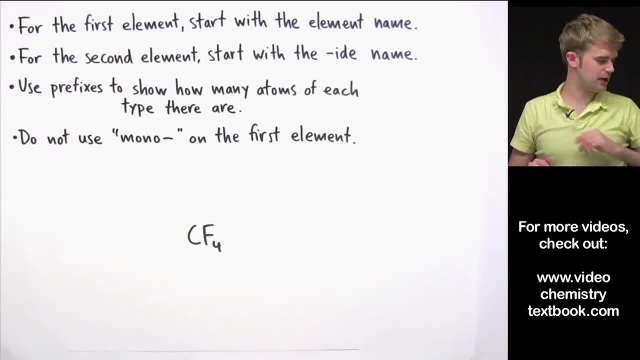 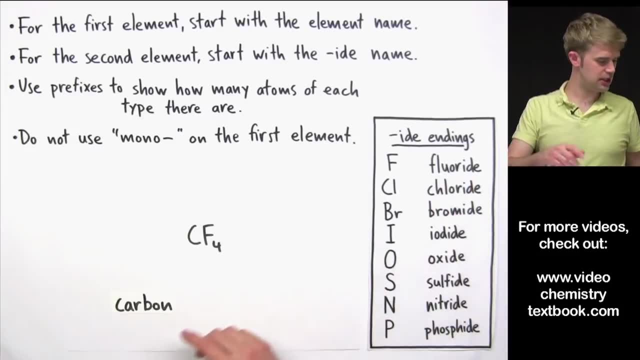 We'll start it off just normally. So, for the first element, start with the element name, That's carbon, And then the second element, which is fluorine, we use the IDE name, which in this case is fluoride. Okay, now we get to the prefix part, and this is where things change a little. 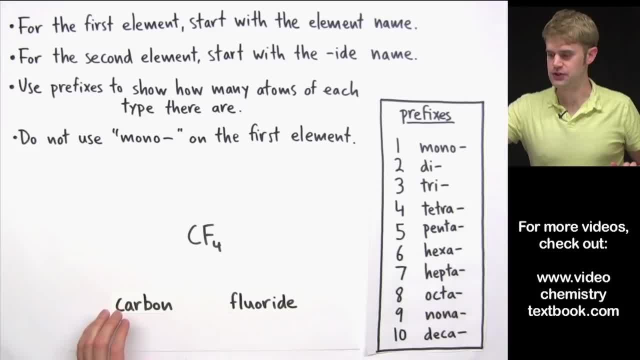 bit. So it says: do not use mono on the first element, Carbon. here we only have one of them. You might want to use mono and put it in front of here. That would be a perfectly logical thing to do. But for whatever reason, we don't use mono on the first element. if there's just one of them, We 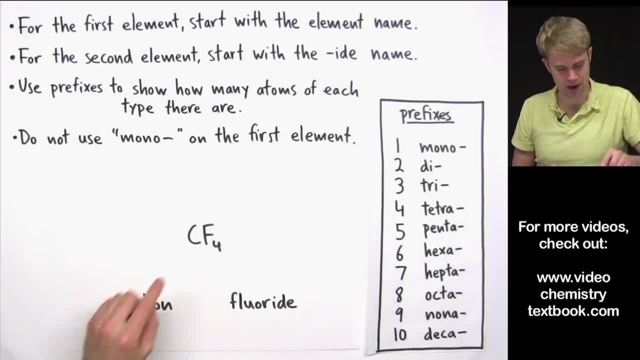 just leave it like this. You don't put anything there. So we have one carbon, we're just going to call it carbon. And then for fluorine, here in front of fluoride I'll put the prefix just like I would any other time. So I have four of these fluorines, So I'm going to call it tetra, Tetra. 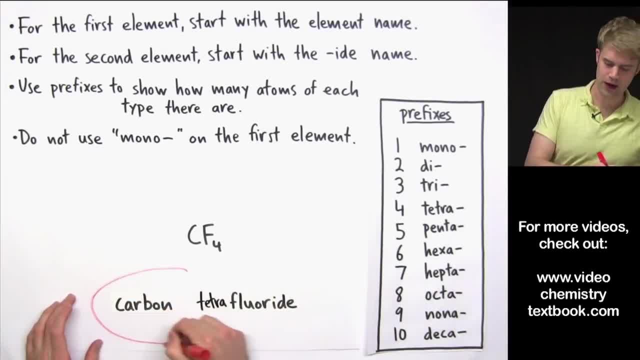 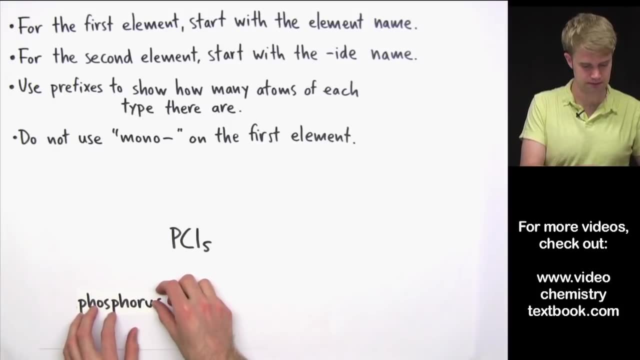 fluoride. So carbon tetra fluoride, not monocarbon tetra fluoride, just carbon tetra fluoride is how we name this, because if you've got just one of the first element, you don't use anything. PCL5, let's name this So P. the first element is phosphorus. Cl. the second element is chlorine. 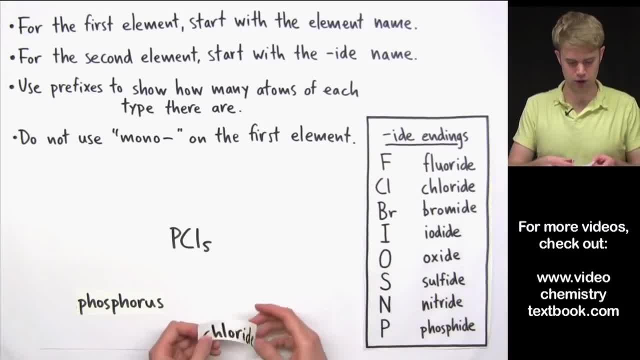 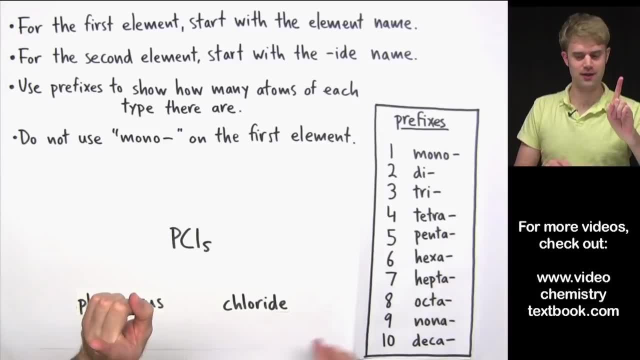 And chlorine's IDE name is chloride. So there it is. Now we get to the prefixes Phosphorus: here we only have fluoride, So we're going to use fluoride. Now we get to the prefixes Phosphorus: here we only have one of them, So we're not going to use mono here. We're just going to keep it as. 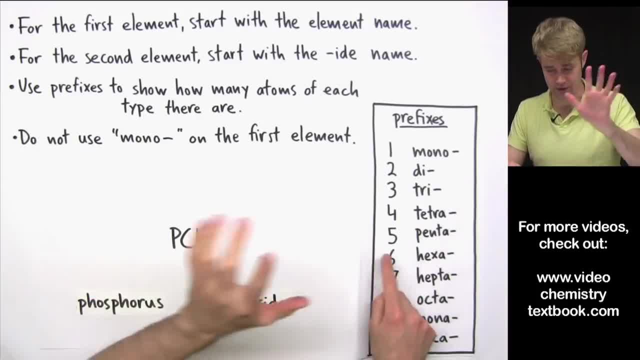 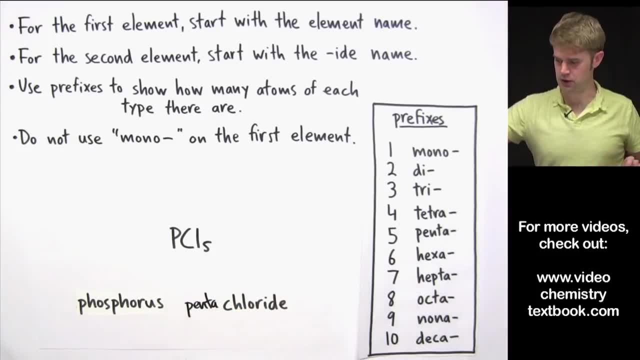 phosphorus And chlorine. we have five of those, So we're going to use penta here as the prefix. So it's going to be penta pentachloride And phosphorus pentachloride, not monophosphorus. 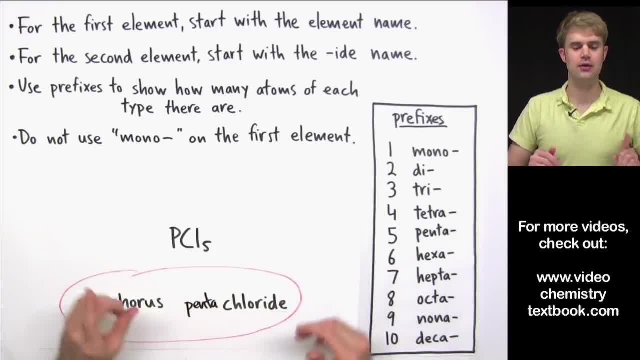 pentachloride, just phosphorus pentachloride is how we name this. Now there's one more step that we're going to add. I'm going to talk about that next. Okay, there's one more step to keep in mind. 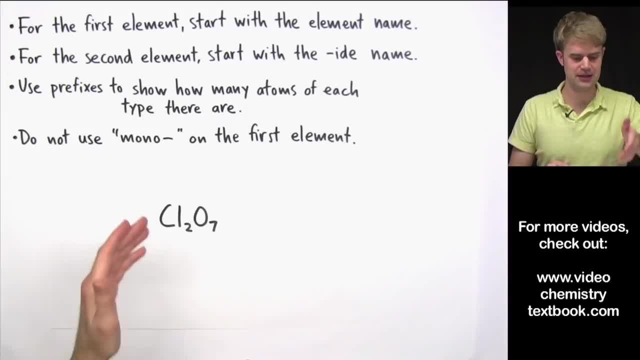 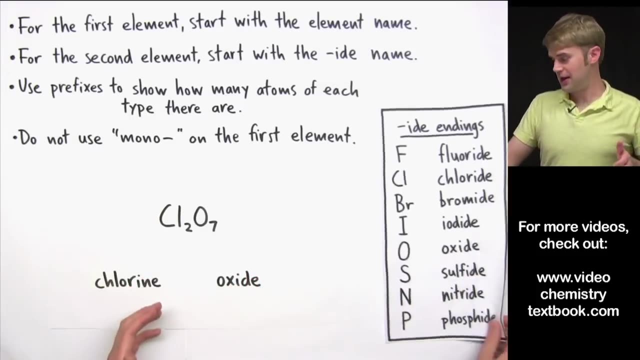 and I'm going to show it to you as I work through this. Okay, CL2O7.. The first element here, Cl, is chlorine, And O here is oxygen. Its IDE name is oxide. Okay, so now the next thing I'm going to do is I'm going to use these prefixes. So I got. 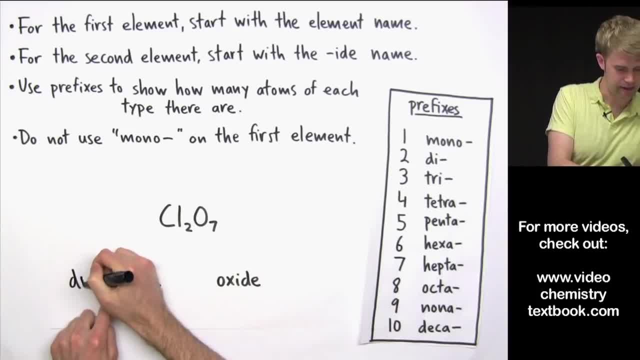 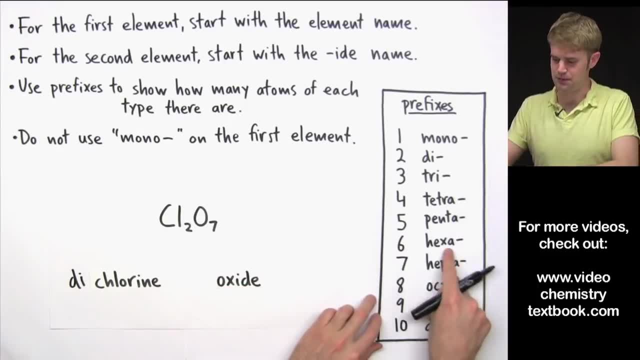 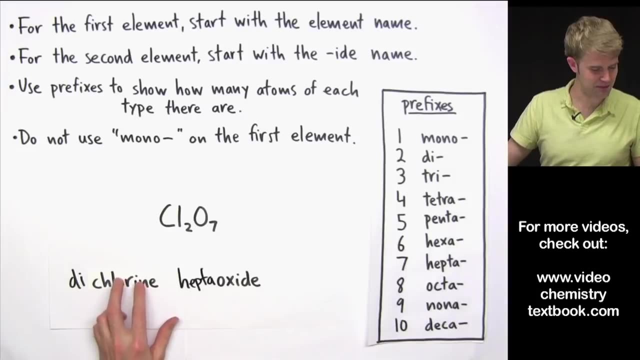 two chlorines, So I'm going to use di Di for two up here, And then oxide. I got seven of those, So I'm going to use the prefix fix hepta. now try saying this compound name. we got dichlorine heptoxide here, that heptoxide thing. 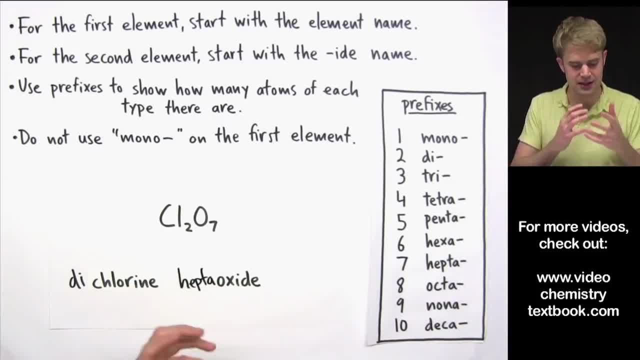 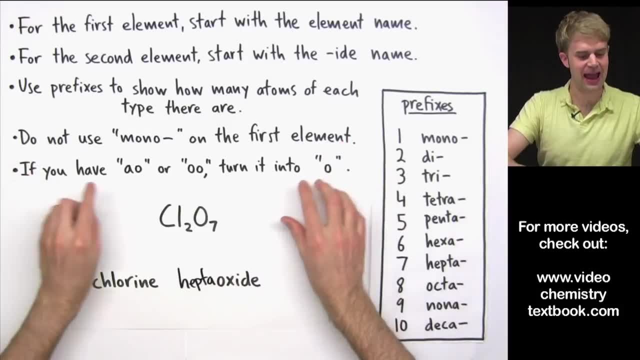 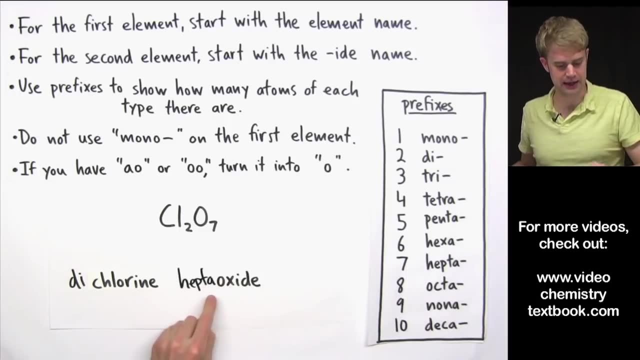 it's kind of awkward to pronounce. so to prevent us coming up with these really weird names, there's one more rule, and that's that if you have a o or o, o turn it into o. here's what that means. we got this heptoxide here, so to make this easier to pronounce, we turn the ao that we see right there. 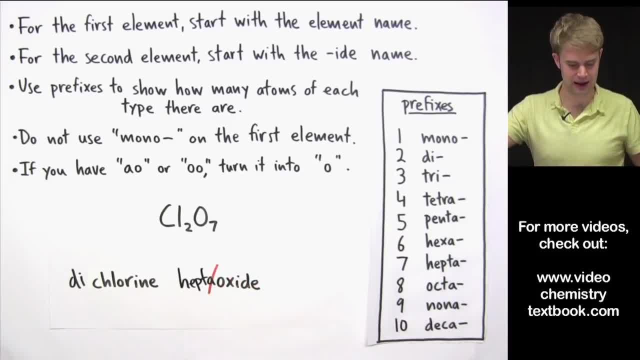 into just an o. so i'm going to get rid of that a. i'm going to get rid of that a and i'm going to turn this compound name into chlorine heptoxide, so not heptoxide, but just heptoxide. so you get rid of that a. if it's next to an o there, let's do one more, p406, so the p. 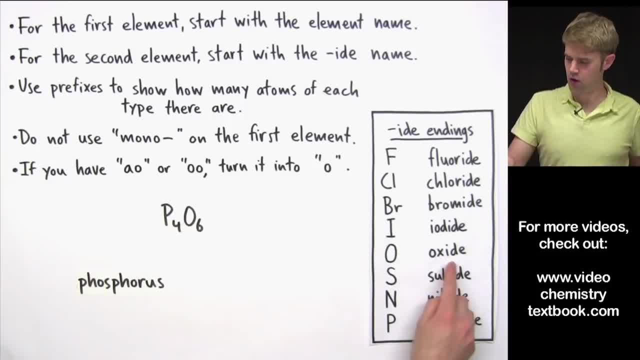 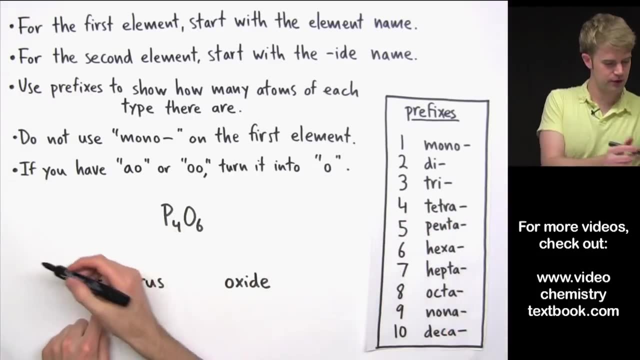 406, phosphorus is our first element, and then o we got oxide. that is the ide name for oxygen here. all, right, now let's use the prefixes. switch to our prefix table. here we have four phosphorus, so we're going to use the tetra prefix, so tetra, tetraphosphorus, and then for oxygen we have six. 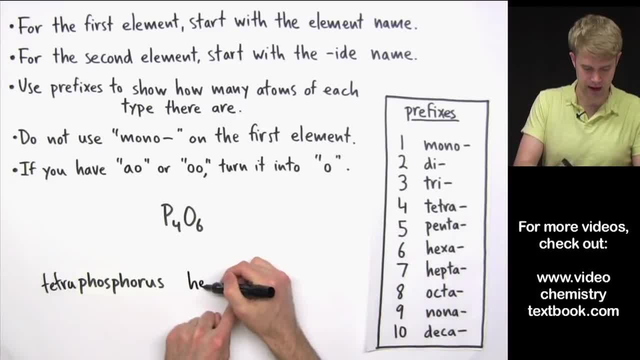 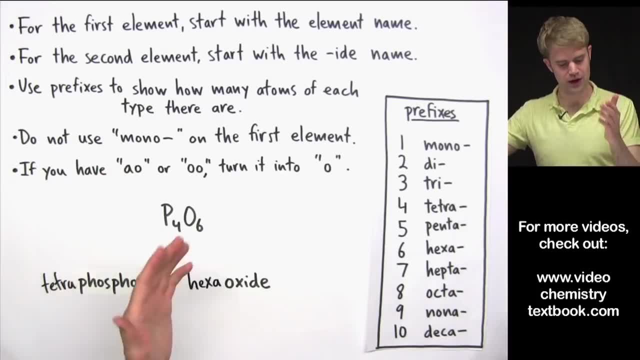 of those. so we're going to use hexa here and, just as before, we end up with this awkward name hexoxide, we get an a oh, so we're going to get rid of this a here, oh. i always like knock that name out of the way. hexa oxide and that turns it into 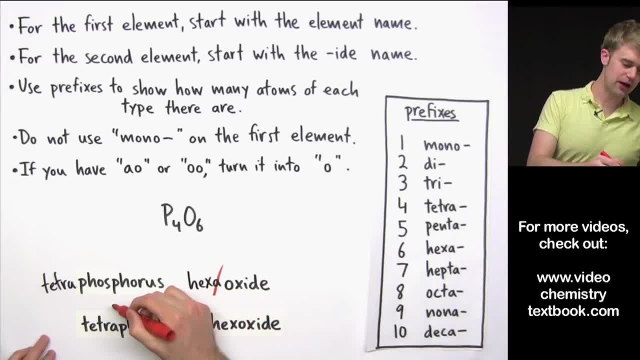 tetraphosphorus hexoxide. you know i forgot to circle the name in the last one and this is just so satisfying so i did it really slowly to make up for the fact that i didn't circle the last one. so we get rid of this. a here: tetraphosphorus hexoxide. here, when you're focusing on谢. 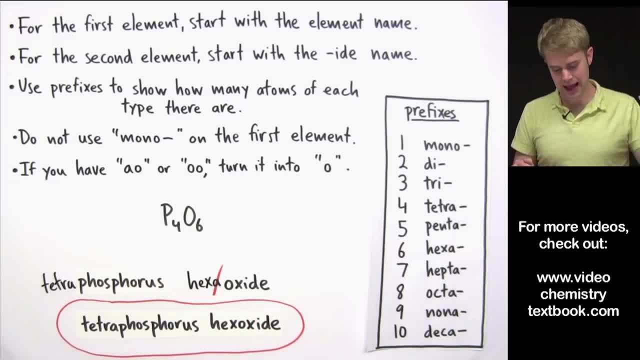 co преп suasos Wide July 2019. So I want to do one more example that pulls in examples of all of this. It's like a good review for all of these things. Here's our last formula: This is a really good review. 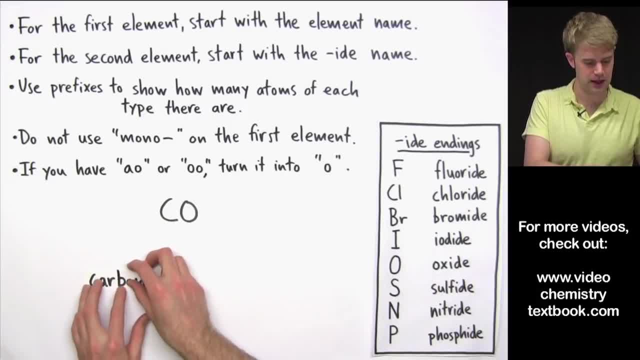 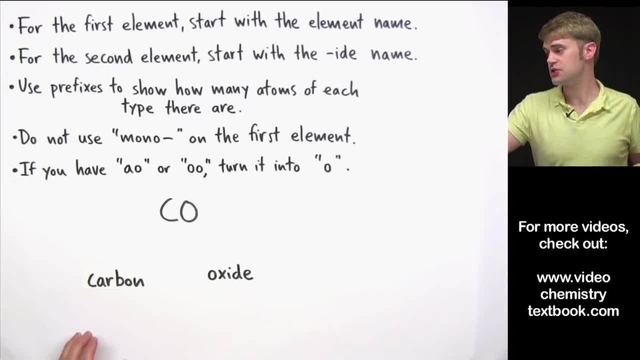 It's just CO. So the first element is carbon, The second element is oxygen. Its IDE name is oxide. Okay, so now for the prefixes Carbon. we've only got one of them, So, remember, don't put anything in front of it. 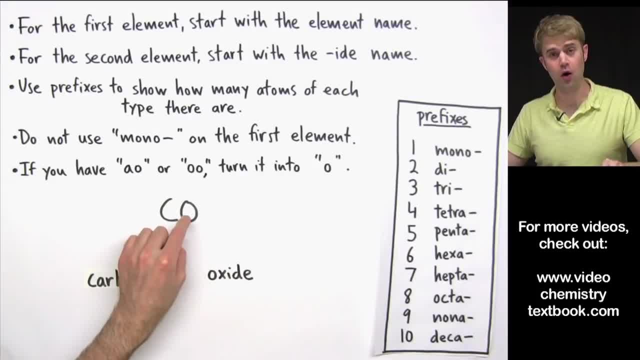 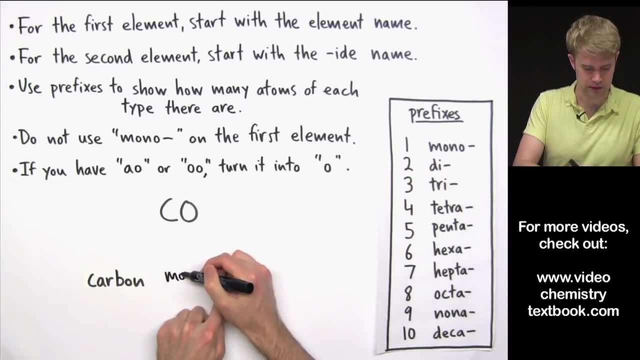 We just call it carbon. But we have one O, and if you have one of the second element you do use a prefix. So we use the mono prefix here. So mono, Now monoxide, gives us this same kind of weird pronunciation thing. 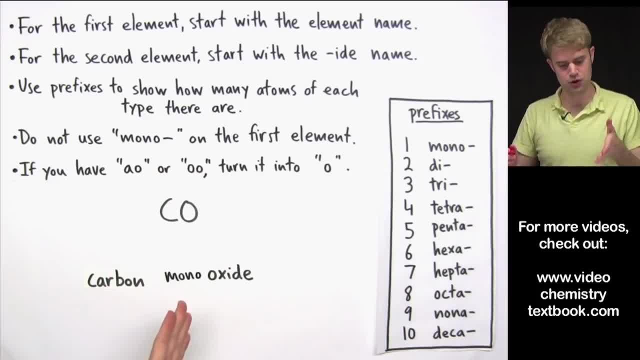 It gives us an OO here, So we're going to get rid of this. Oh, I'm going to try to not knock this name out here. Oh, just a little bit, Really good, And we call this. we change the name from monoxide to carbon monoxide. 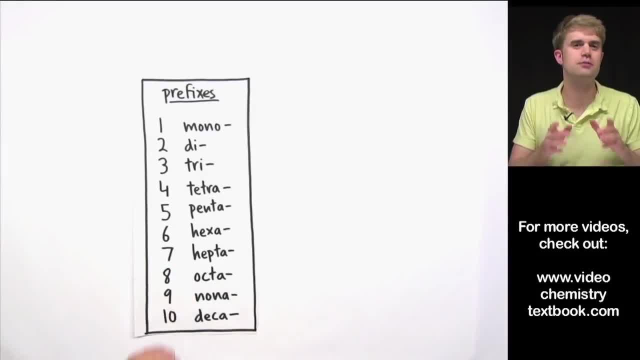 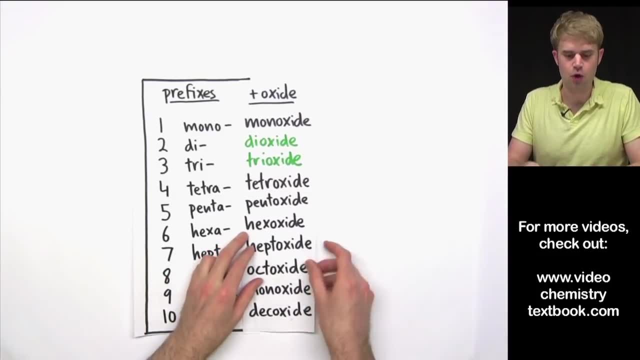 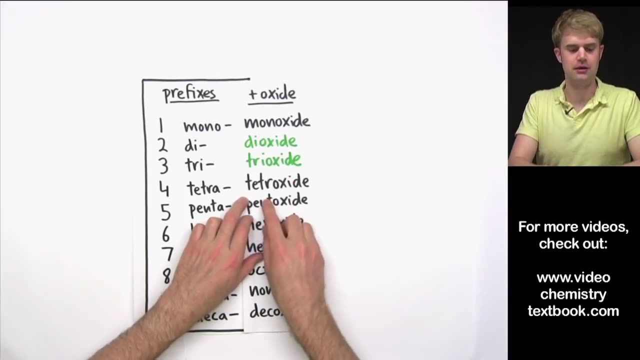 which is probably That's something that you've heard of before. Here's just some quick information about how we change these prefixes to avoid an awkward pronunciation problem. We only really have this problem with oxide because it begins in O, And so we get rid of the O here in mono and we get monoxide.